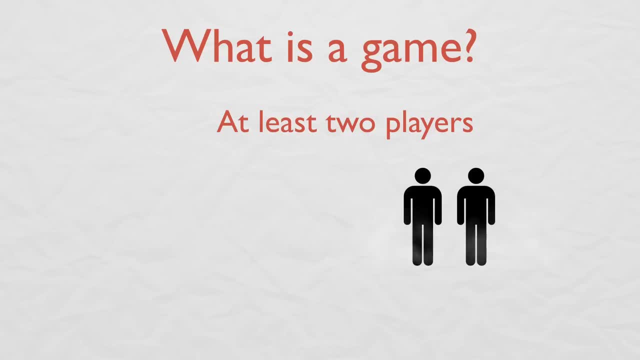 or if you want to be really crazy people And you need payoffs for the players, You need to define the outcomes they can potentially get, depending on how the game unfolds, And, finally, you need rules for the game. Now, it's not always obvious how people will behave. 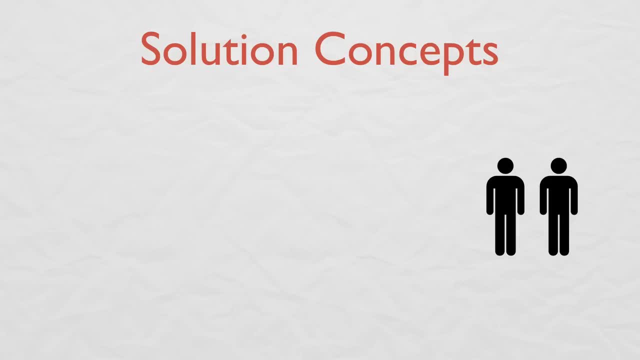 even with players, payoffs and rules clearly defined. That's why game theorists have a number of solution concepts for games, including the dominant strategy equilibrium, the Nash equilibrium, the sub-game perfect Nash equilibrium, the Bayesian equilibrium and the weak perfect Bayesian equilibrium. The most basic solution concept is the dominant strategy equilibrium. 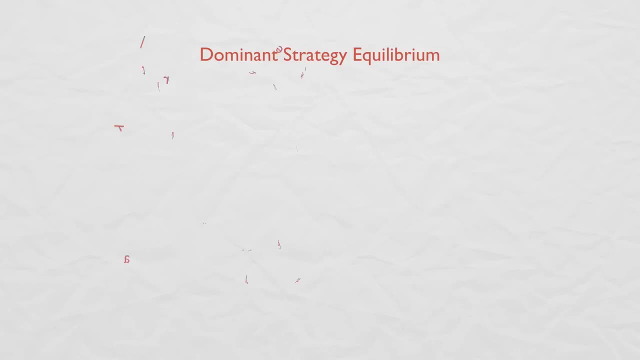 In a game, each player can have any number of possible strategies. One strategy strictly dominates another strategy if the player is always better off under that strategy, no matter what other players do. If one strategy strictly dominates every other possible strategy a player could take, that strategy is a strictly dominant strategy. We have a dominant strategy. 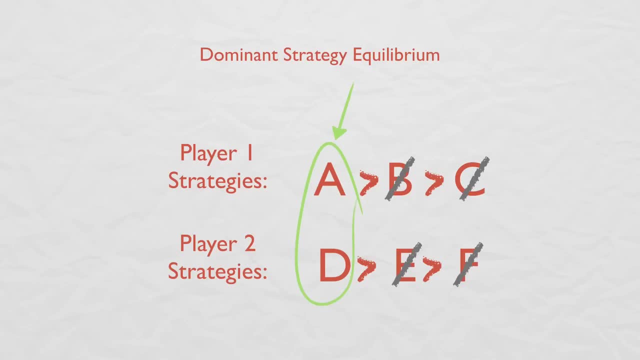 equilibrium. when all players play a strictly dominant strategy, The dominant strategy is a strictly dominant strategy. Now let's look at the most famous game in game theory: the prisoner's dilemma. There are two prisoners, prisoner one and prisoner two, and they each have a choice: They can testify against the other or they can keep quiet. 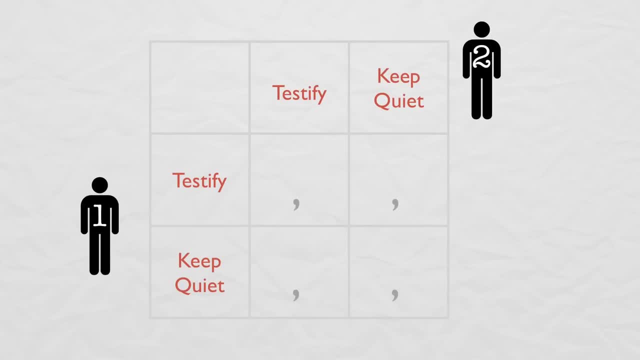 If they both keep quiet, they both get off with a light sentence, which I'll represent, with a payoff of two Prisoner. one's payoff is on the left, prisoner two's is on the right. If they both testify, they both get a moderate sentence. I'll represent the moderate sentence. 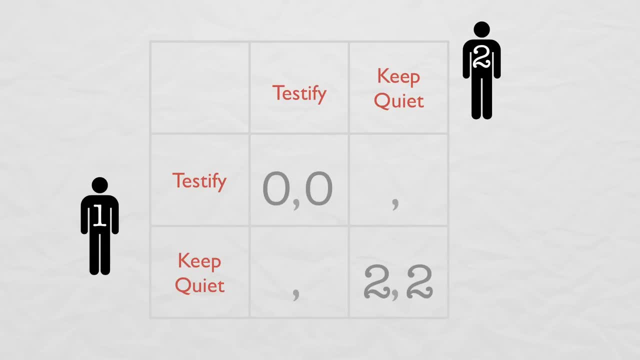 by a payoff of zero. Right about now, keeping quiet is looking like the best option, but there's more to this game. If one testifies and the other keeps quiet, the one who testified will get off scot-free and the one who kept quiet will get an extremely harsh sentence. 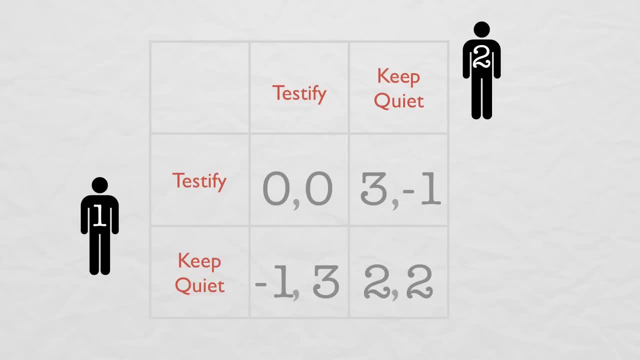 They'll throw the book at him. Think about this game for a moment. Keeping quiet looks like a pretty good option if both prisoners could promise not to testify. but these prisoners only care about their own self-interest, So both prisoners may tell the other- they pinky swear- not to testify.